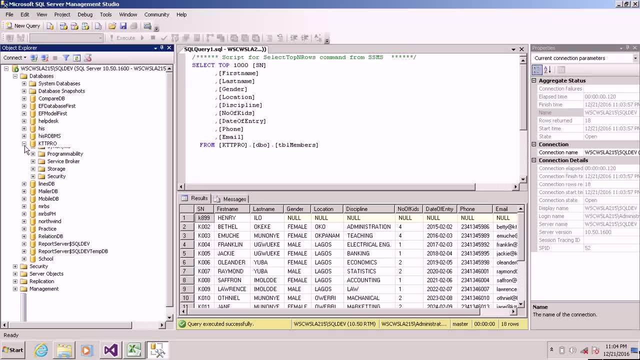 In word re-user, you actually need to review your database. So what you'll do is just click on your database, expand it and then go ahead to expand program ability and then the first one there is stored procedure. If you expand it, you find out that you. 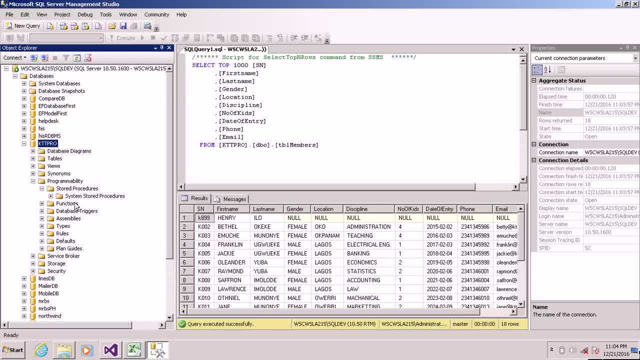 don't have anything except system stored procedure. So what do you do To create your first stored procedure? just right click and then select new stored procedure. All these are very confusing, a whole lot of crap. So you just check and paste and you're done. Copy from your database and then click on Restore to name your database. It's just a drop down, So you have to do a couple of things there. First of all, having a server and the system is not good. That's not good. 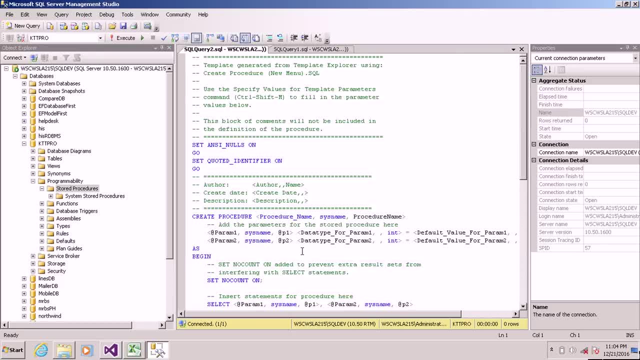 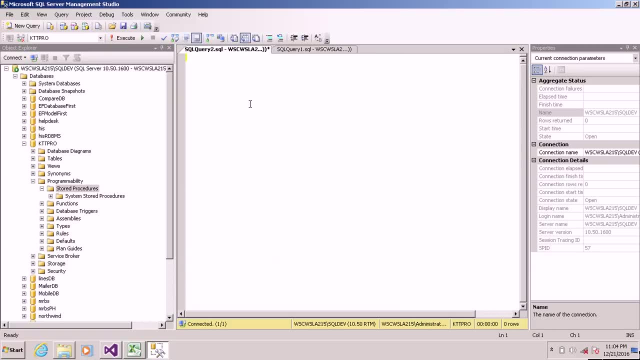 It's not a good thing for customers, so I'm gonna have to change that You need to use to have the production data confusing. there are a whole lot of crap, so just go ahead to select everything and delete, and that is it. so let's write our first thought procedure. take note of the syntax. you simply say: 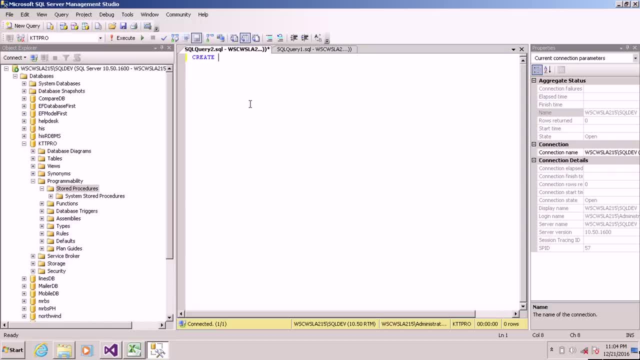 create a procedure and give it a name. let's call it uh first. okay, let's just call it get all members, and then you say us, after you enter us, then you write your query. that is as simple as that. so let's just say: select star from tbl members. so if you execute, good, so you have created this. 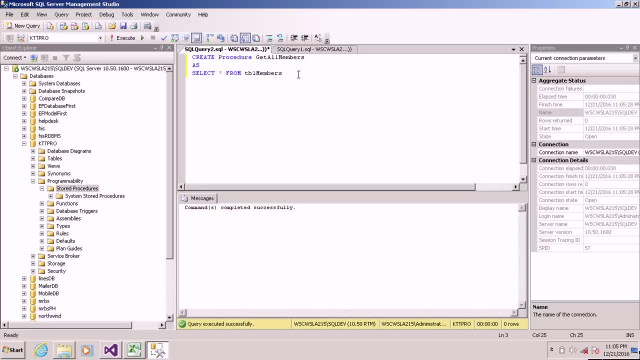 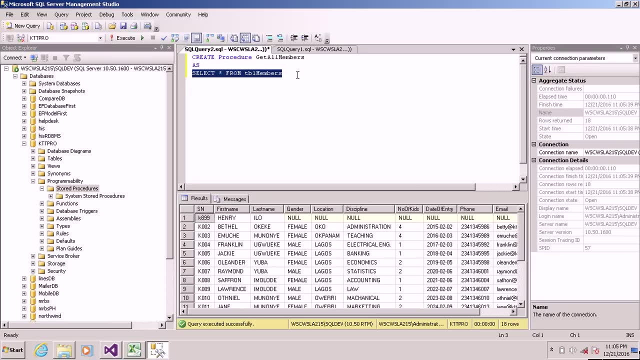 start procedure so it doesn't execute as a query. but if you go ahead to highlight just the query there and execute, it actually executes and gives you what you want. but now we've executed this create start procedure statement so let's go ahead to check. so just do a refresh here, refresh and then expand you. 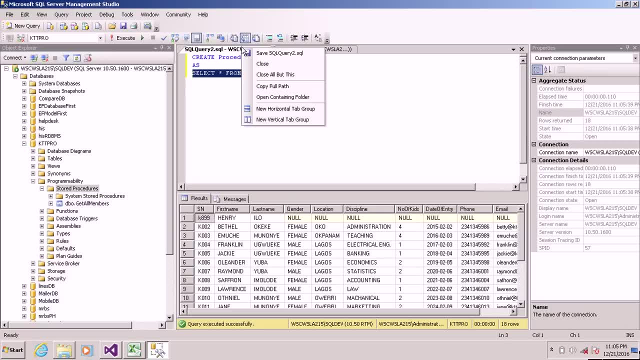 see: uh, get all members start procedure. how easy is that? so that is so fine. the next thing we are going to do is to write a start procedure that actually takes a parameter. let's assume you want to update the start procedure, so let's go ahead and do that. so let's go ahead and do that, so 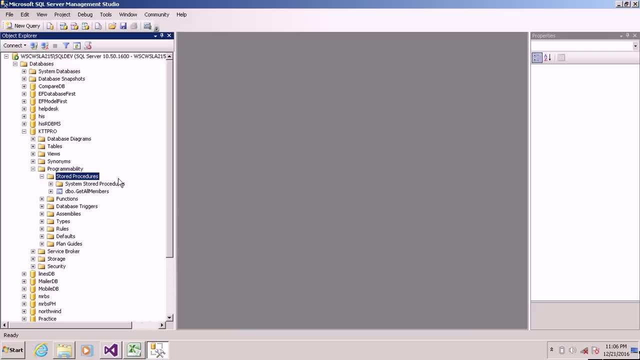 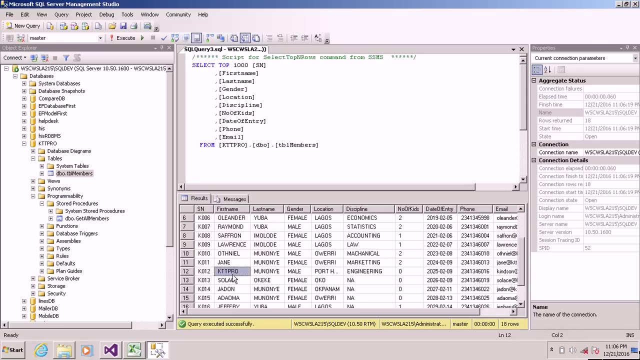 update my name or my son name to something else. let's look at our data again so that we'll be able to make updates. this time we are writing a stock procedure that will accept a parameter. so let's see. you see, ktt pro is a full name, and now i'm going to write a stock procedure that takes a first name. 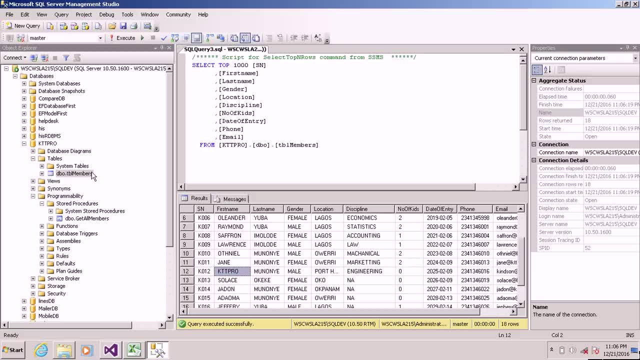 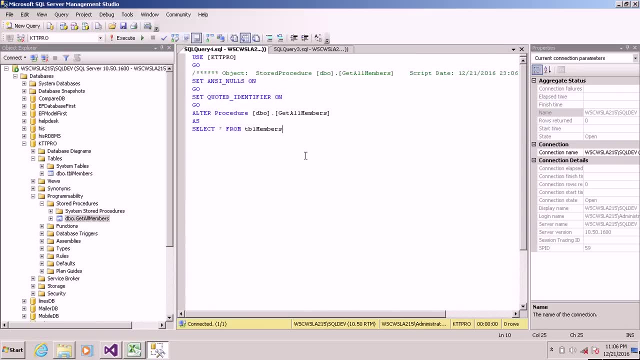 and then changes the ktt pro to something else, so it follows the same. what i normally do is to open existing start procedure by right clicking and say modify, so it adds all this junk might either leave it or you can just delete it. for me i like deleting them. 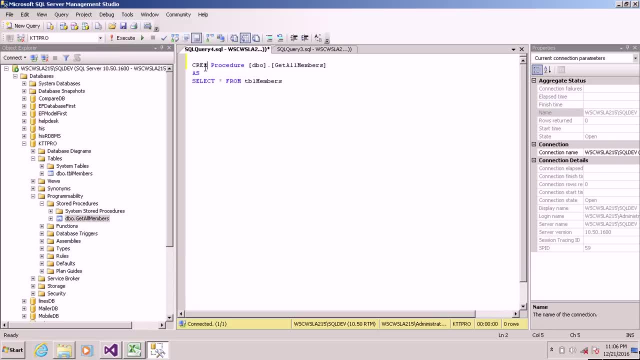 to avoid confusion. so all the statement changes to create because we want to create a new one. we say updates member, but this time uh. the name of the start procedure is update member. before the as before the ask keyword. just say uh and just just specify the, the parameter you want. 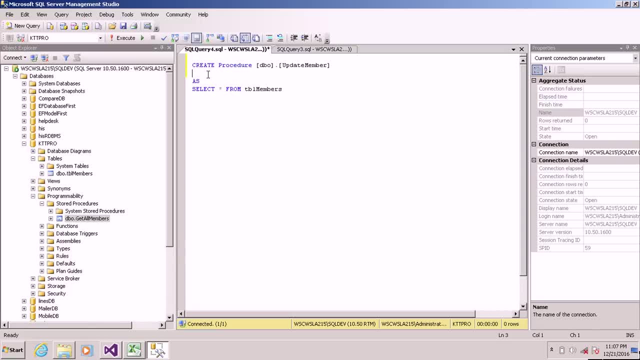 to use, or just like the, the function, the, the arguments, the start procedure. so let's say our first name. take note that always use ads to start the variable name at first name: vodka 50, okay, vodka 50. and then we want to make updates. so of course you know how to write up this statement. 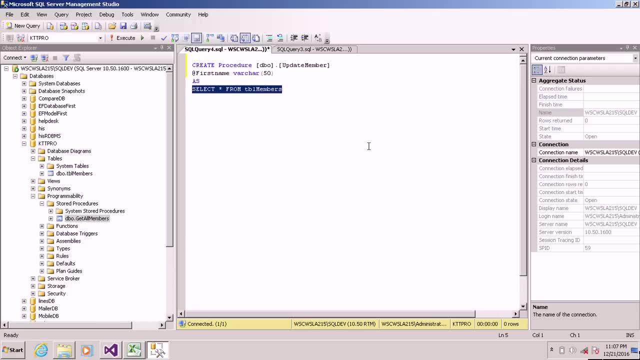 if not, just look at the previous video from the link in the description below so that you'll see how to write queries. so you just say updates, tbl, members, sites, sites. first name equals at first name. take note: at first name is different from from first name. at first name is a parameter. 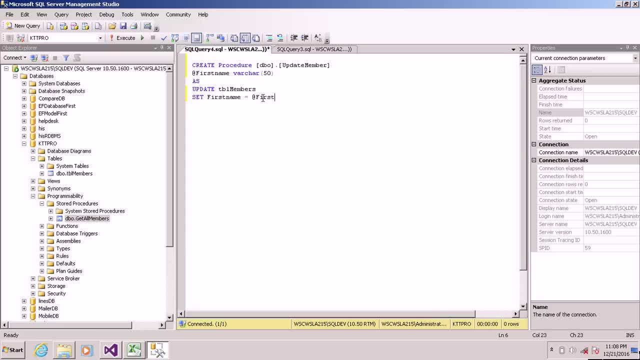 that has to be provided by the user at first name. where we have ktt pro, where first name equals ktt pro. if i'm too fast, please pause the video or just rewind it. so at this point we have a start procedure that says update member and I'm going to execute it and command completed.